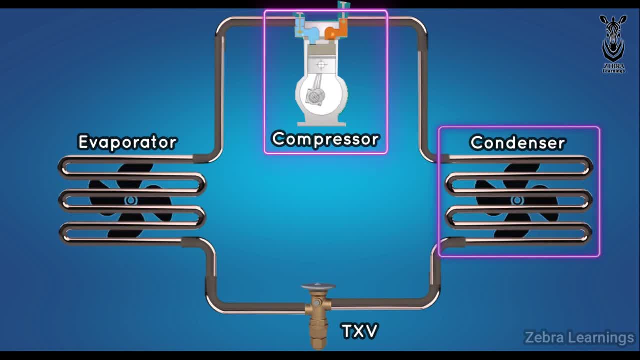 They are: compressor, condenser, expansion valve and evaporator. First, let's see from the compressor. The compressor increases the pressure of the refrigerant. By increasing the pressure of the refrigerant, the refrigerant can travel throughout the cycle. 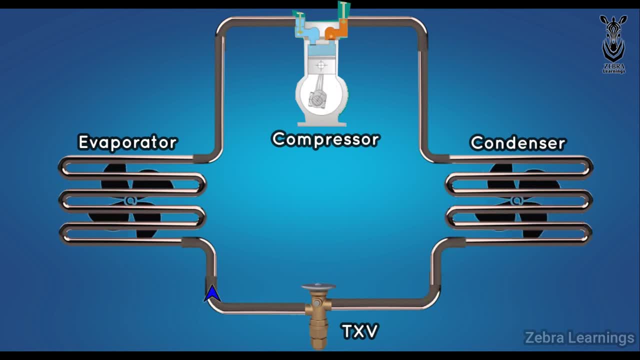 In the compressor. the anticipating method is: which external heat leaves is duration of coolant. As a result, the crystallization is stimulated. Refrigerant enters the compressor at low pressure, low temperature and vapour state. The compressor compresses the refrigerant well and sends it out. 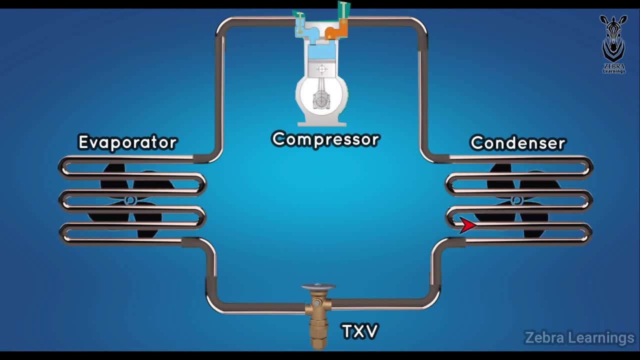 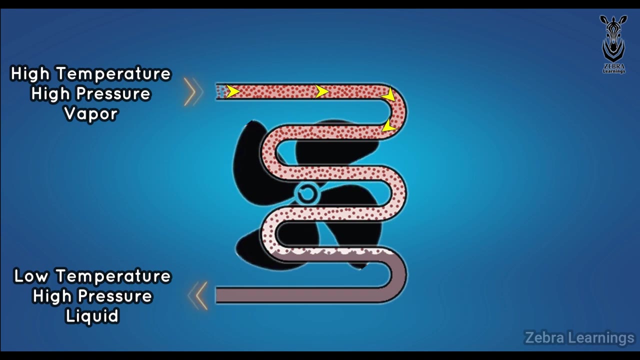 When it comes out of the compressor, the refrigerant is at high pressure, high temperature and vapour state. The refrigerant goes to the condenser. Condenser coil is a heat exchanger in the refrigeration cycle. The condenser coil cools the refrigerant coming from the compressor at a high temperature. 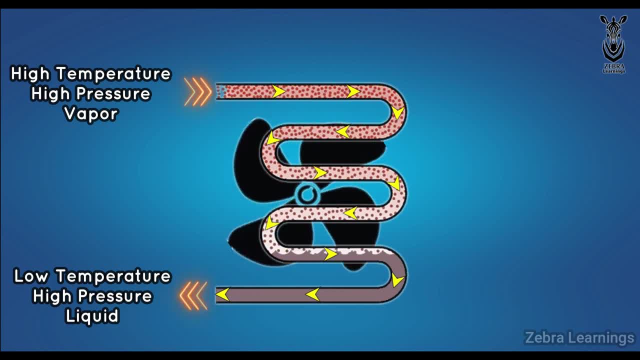 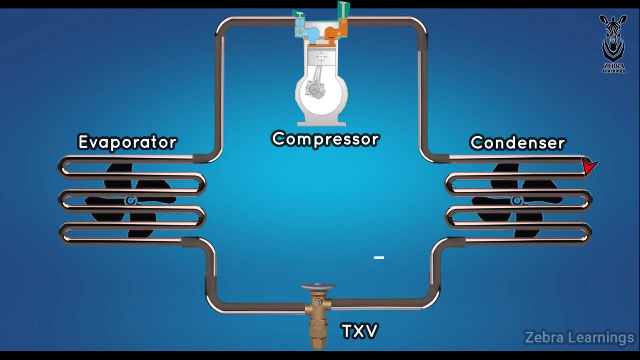 As the heat in the refrigerant is released, the refrigerant changes from vapor state to liquid state. It now comes out of the condenser at high pressure, low temperature and in liquid form. Next the refrigerant goes to the expansion valve. 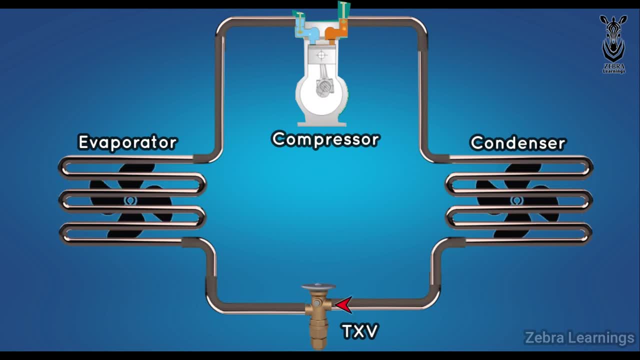 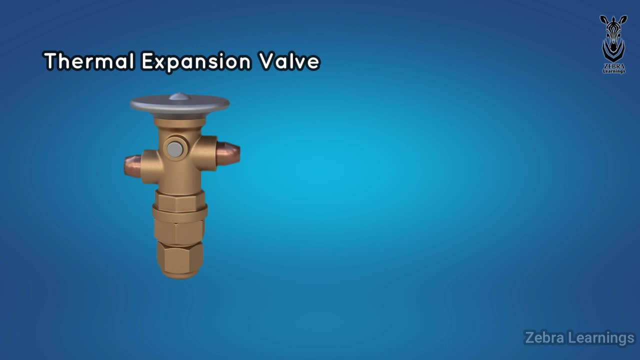 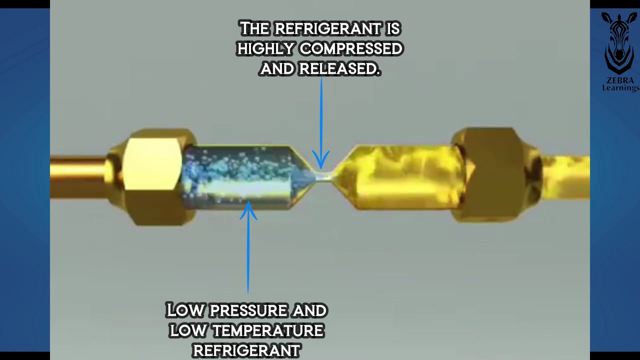 Although there are many types of expansion valve, thermal expansion valve is mostly used in many places. The most advanced of these is the electronic expansion valve. But whatever the expansion valve is, its important job is to reduce the pressure of the refrigerant that can come from the condenser at high pressure. 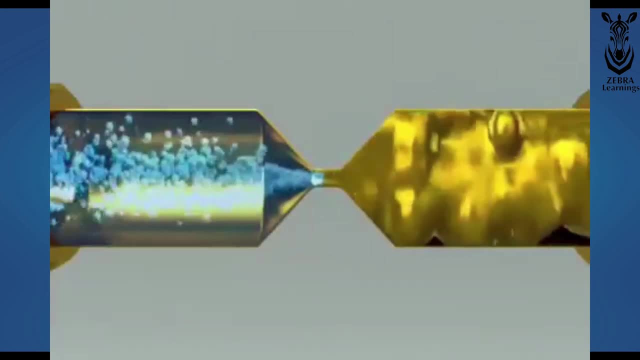 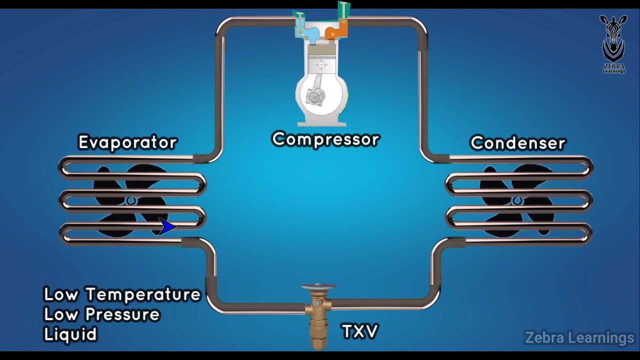 By reducing the pressure, the temperature of the refrigerant will decrease. The refrigerant that comes out of the expansion valve at low temperature, low pressure and liquid state then goes inside the evaporator. This evaporator is another heat exchanger In the refrigeration cycle. refrigerant enters it at low temperature, low pressure and liquid state.